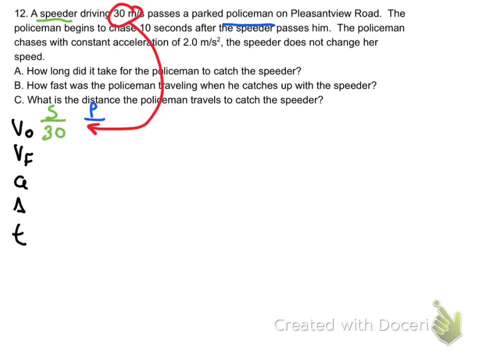 The speeder's initial velocity starts the problem, moving 30 meters per second. and the police car is parked, so its initial velocity is zero. The speeder goes 10 seconds, while the police car is waiting to chase. so the speeder's going 10 seconds longer. so it gets T plus 10, while the police car just gets T. 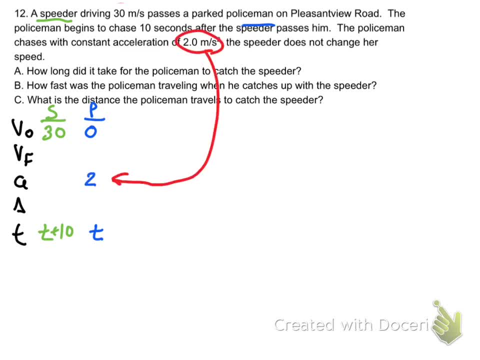 It says that the police accelerates at 2 meters per second squared, and it says nothing about the speeder's acceleration. so the speeder gets a zero for acceleration. So we have two columns, one for the speeder and one for the police, since we have two objects moving in this problem, and we lay down our variables: V0, V, final, A, delta and T. 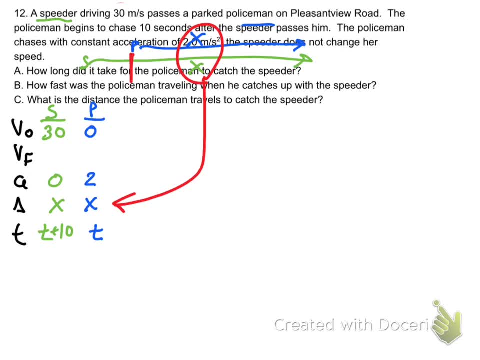 Then we look at how far they traveled. The speeder's, moving along, reaches the police car. that's when our problem starts. and then the police catches up to the speeder so they both go the same distance. X during our problem. 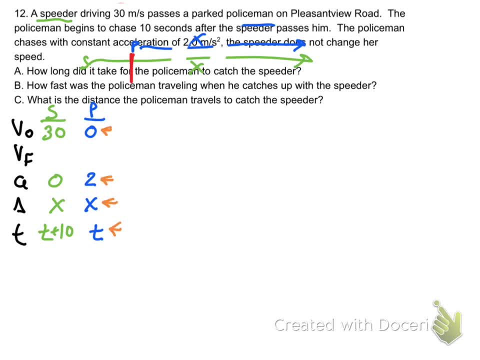 We look at the variables we have. We have V0, acceleration, delta X and time and we have to find the equation that relates them, And that's: delta X equals V0, T plus one half A T squared. 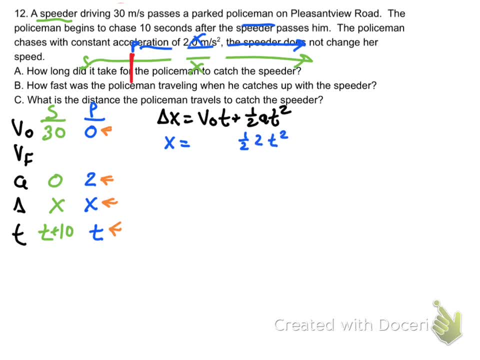 We do the delta X equation for the police car. The police car's initial velocity is zero, so that term is not in this equation. And we do the equation for the speeder where we have initial velocity times time. The speeder does not accelerate, so that term is not present. 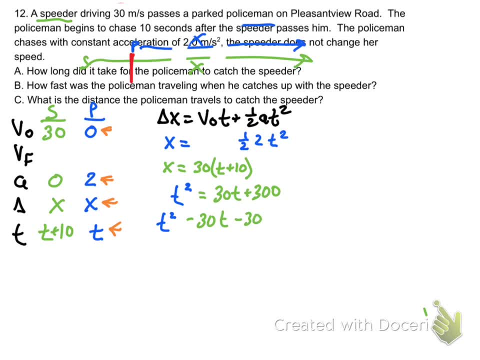 Since both of these X's are equal to each other, we can set the right-hand sides equal to each other. And don't forget to distribute that 30 times the T plus 10 to get 30T plus 3.. Now we have to do the quadratic expression to find out what T is. 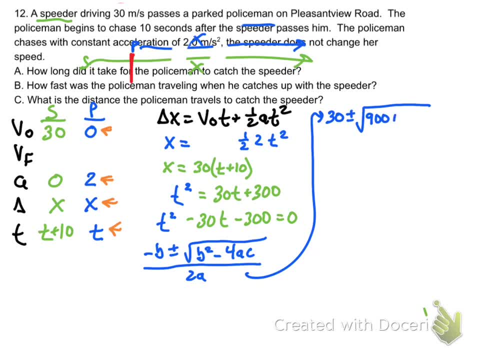 So we go through, we do our algebra: B squared is 900, 4AC is 1200, all over 2A, which is 2.. Then I like to evaluate inside the radical, and that's 2100, and the square root of 2100 is 45.8.. 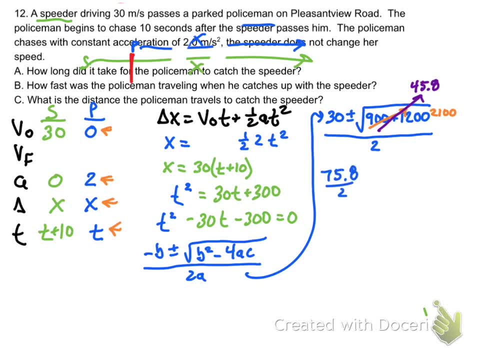 Now we do 30 plus 45.8 and get 75.8 over 2, and 30 minus 45.8.. Gives us negative 15.8 over 2, but we don't want the negative root so we use the positive root, which is 37.9 seconds.